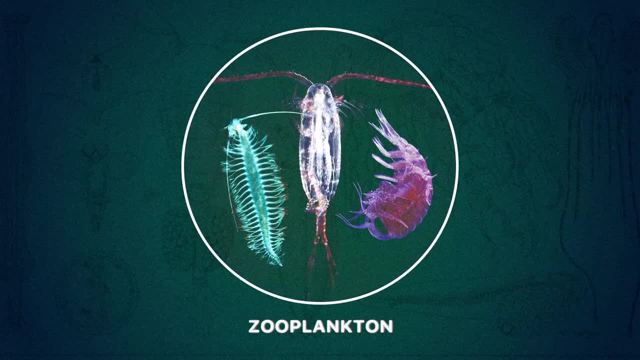 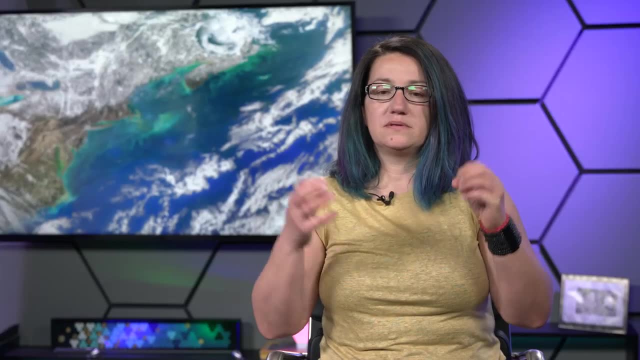 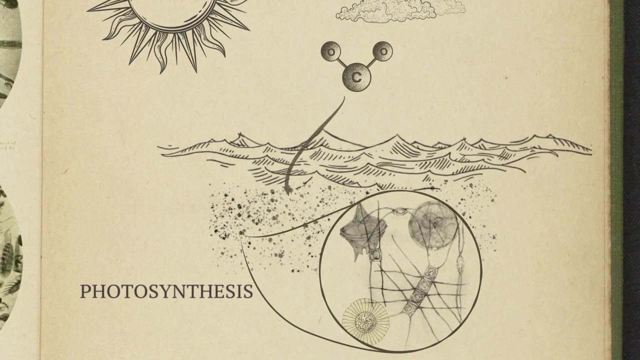 Plankton we can define traditionally in zooplankton, so something that is kind of more animal-like, And phytoplankton something that is more plant-like. All phytoplankton does is what we call photosynthesis. They take carbon dioxide and carbon in organic form, capture some of the sunlight and then produce carbohydrates or, just simply said, sugars. 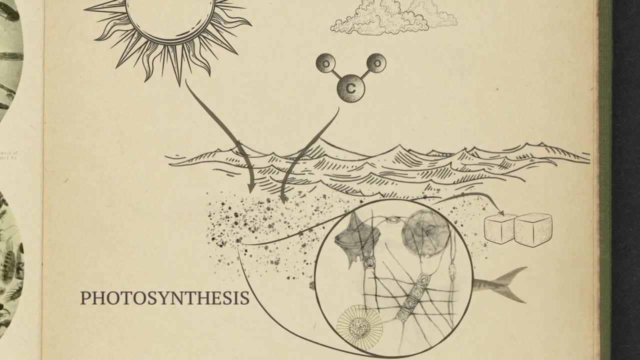 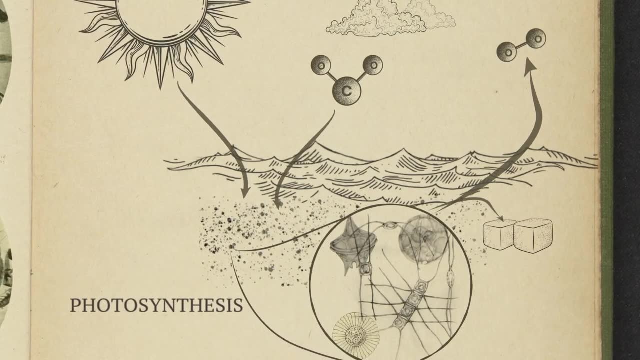 They now are carrying that sun energy and push it into the food system of the ocean, And while they're doing all that stuff, they also produce the oxygen. So, opposites from us, We inhale oxygen, exhale carbon dioxide. So that's why they're really important. That's why we love them. We love them so much And that's why they're, like, really crucial for the whole life on the Earth. Phytoplankton itself: its diversity is gigantic. I think there's like 10,000 species, and each of them has a specific role. 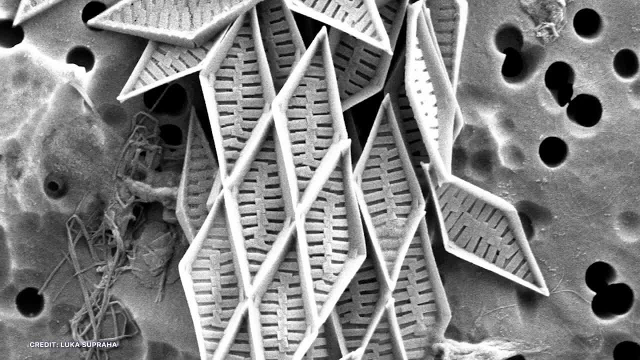 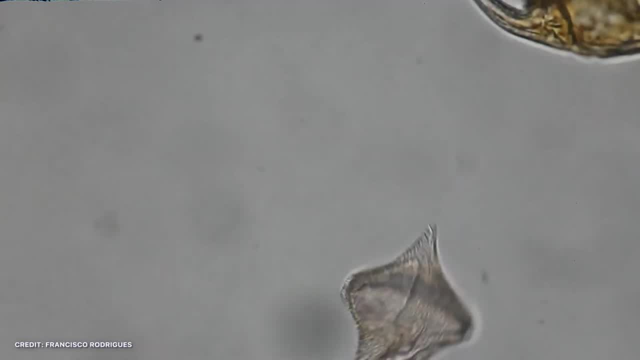 Why is there so much diversity in something that is so teeny tiny? It's fantasy, science fiction and horror comes together. I mean, it's just so beautiful. But there's a certain type of phytoplankton called coccolithophores. 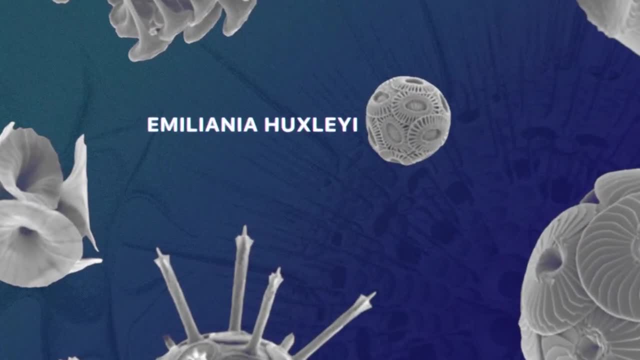 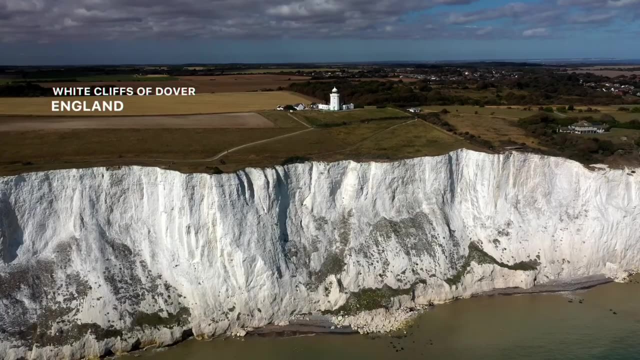 And specifically the most famous one is the Myliania huxleyi. But they take this inorganic carbon to make that something like a shell in which they live in Their calcium carbonate which they make, which is pretty much chalk. they make it in the shape of these hubcaps. 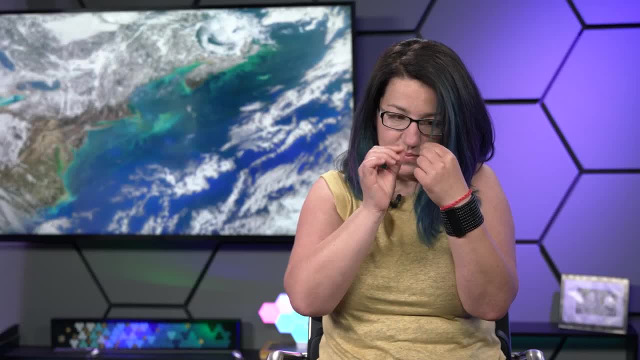 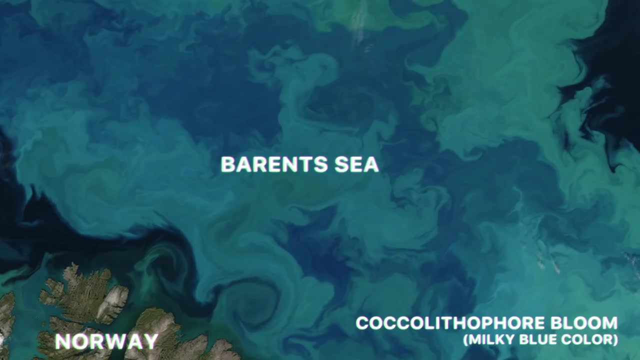 And if you think about how teeny tiny they are, they're like you know, I don't know. I can put probably like 30 or 40 or 50 of them in the width of my hair When they bloom. once they die, not only do they take that, 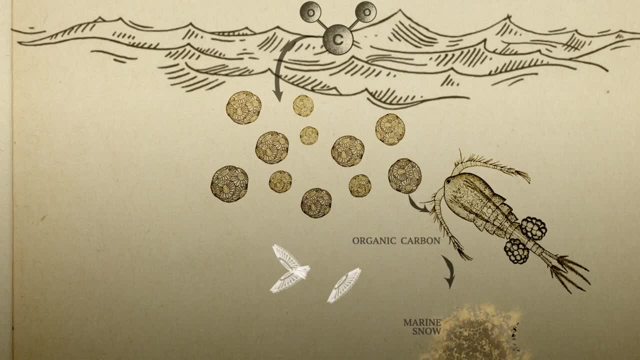 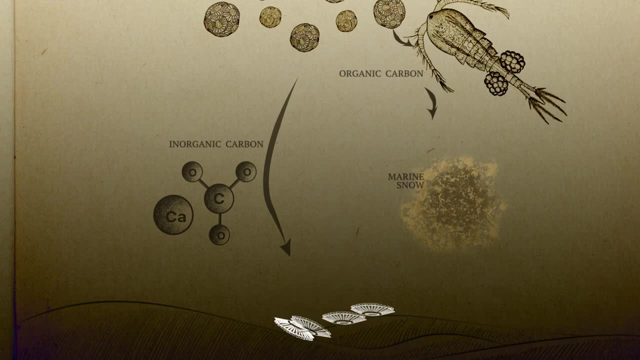 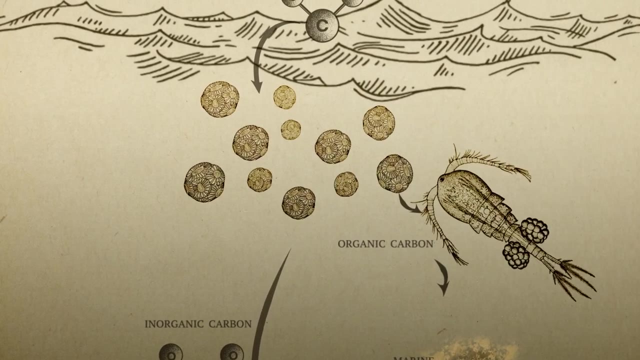 Normal, like sugar carbon that they produce, but they also take that calcium carbonate, that inorganic, that chalky material down to the bottom of the ocean. So they're really, really good for exporting carbon, removing it from this, this contact with the atmosphere, which is really important when it comes to the flow of carbon in the whole, you know, Earth ecosystem, but also control of the carbon in the atmosphere. 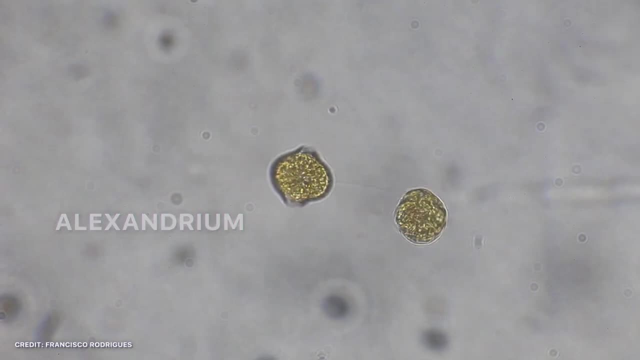 So Alexandrum is a very specific type of phytoplankton. It's called a dinoflagellate. So it's kind of like maybe plant, maybe zooplankton, maybe it's animal, maybe it can be both, you know.